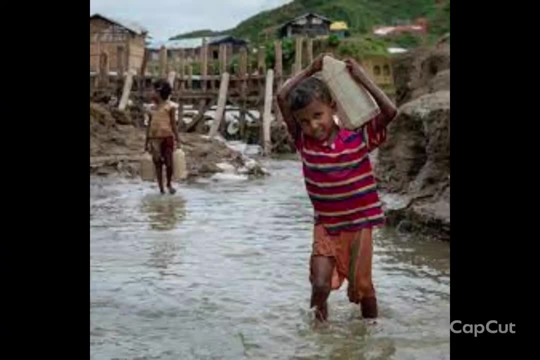 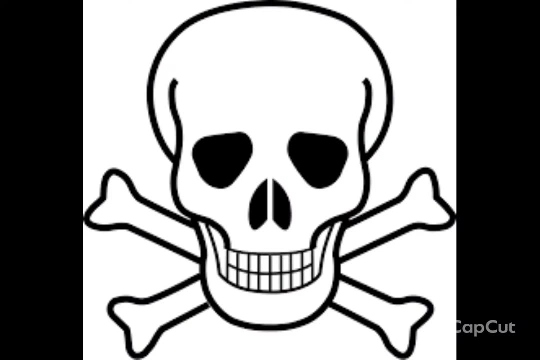 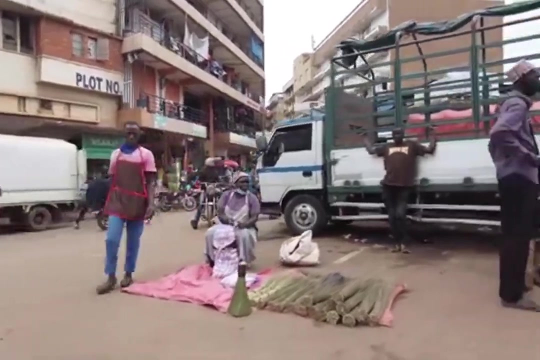 water. This means they rely on untreated water that has not been separated from human sewage, which can cause illnesses and death from diseases such as diarrhoea. Eritrea: 80.7% of Eritrea's residents lack basic clean water services. The population: 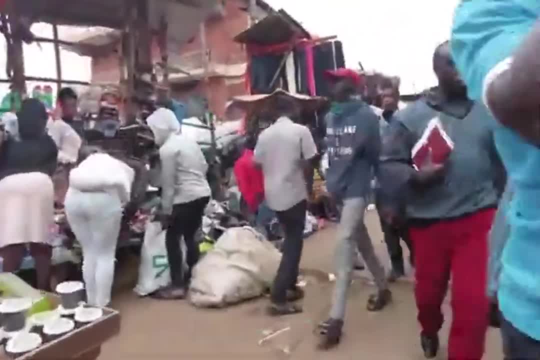 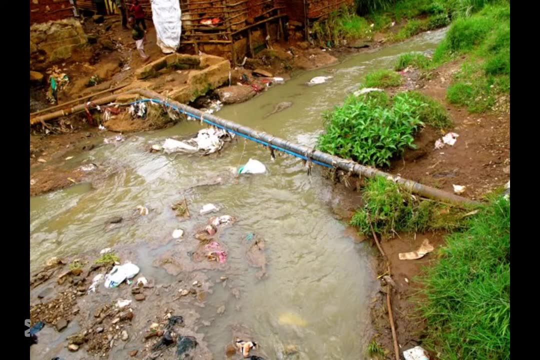 of Eritrea in east Africa has the least access to clean water close to home. Lack of household sanitation means open water sources are often contaminated by human and animal waste. due to the heavy pollution of water, Eritrea is the only country in the world that has a high 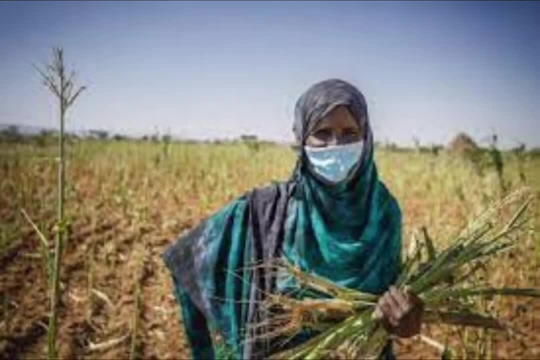 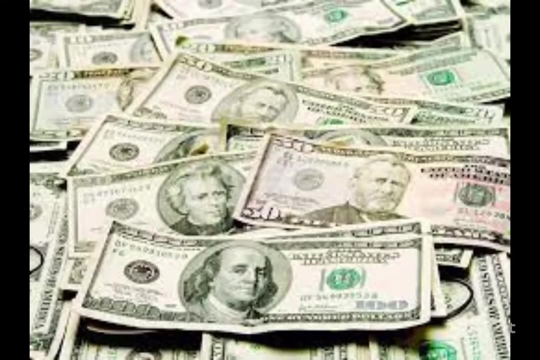 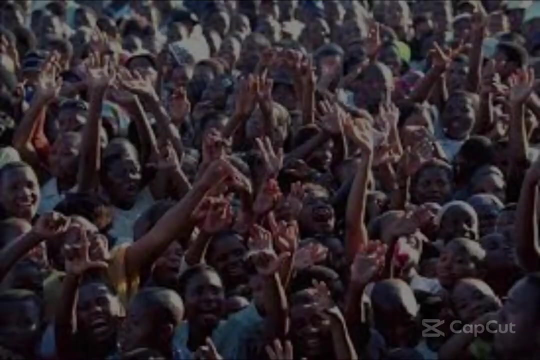 poverty reliance on agriculture in Eritrea and the already unreliable rainfall. The addition of drought to such a region is catastrophic. When the main source of income for many is impacted, the poverty rates increase and the economy begins to crumble. The population of Eritrea is a problem. 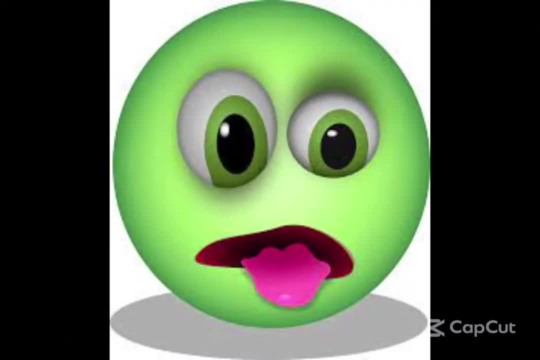 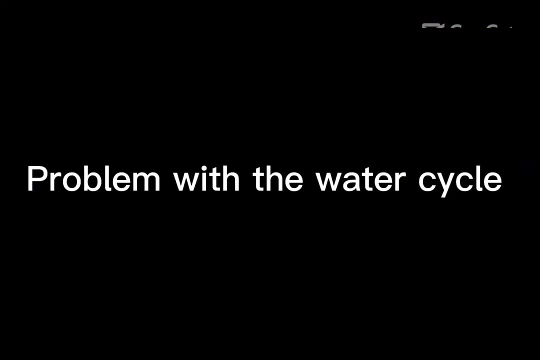 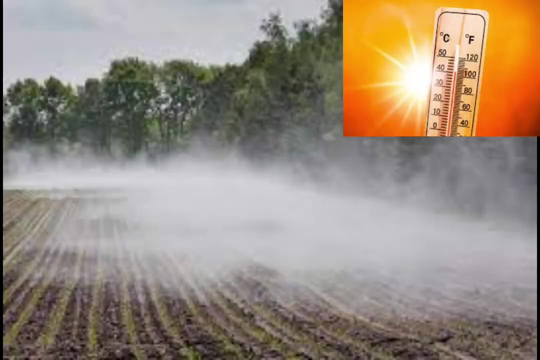 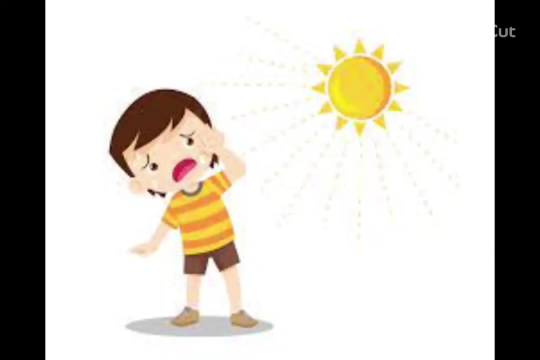 for the water supply, as most of the water is contaminated. They have to share the clean water with 6.081 million people. The lack of water is really poor and is worse with a very dry climate. The evaporation rates are much higher and this causes most of Eritrea's water to evaporate. 70% of Eritrea is hot to very 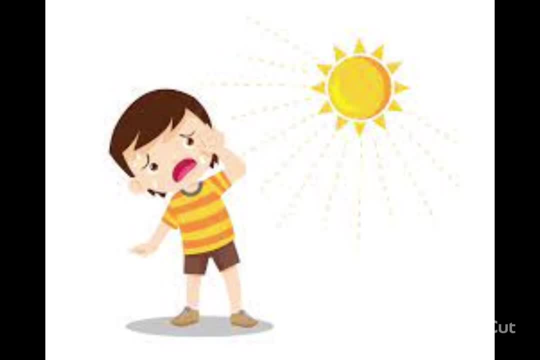 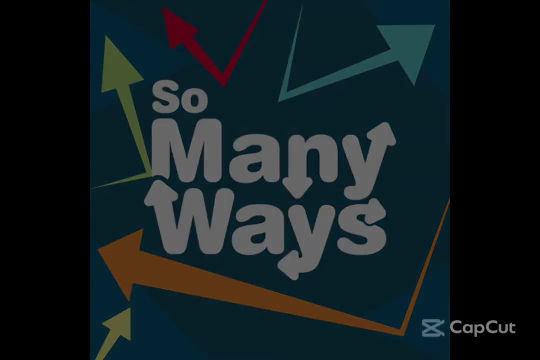 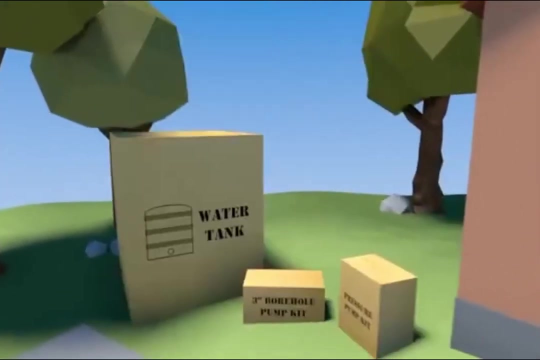 hot, meaning annual temperature is more than 27 degrees Celsius. There are many ways to improve access to clean water. Water borehole drilling is a form of water well drilling. Essentially, it involves drilling a hole deep into the ground to access the water below. 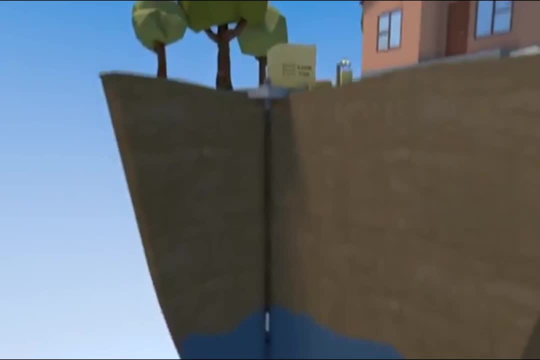 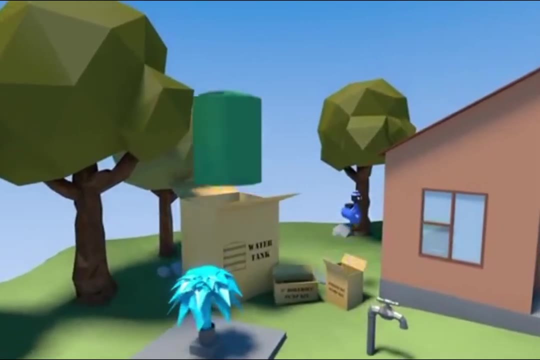 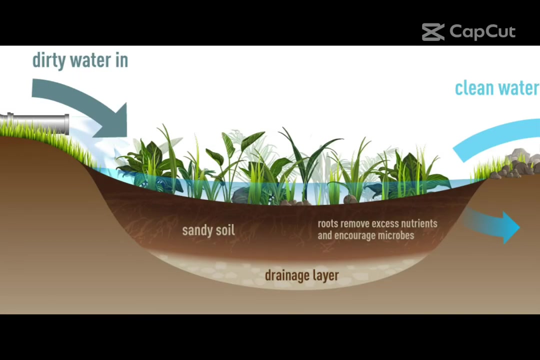 Installing steel casing in a borehole pumping system then enables you to extract natural water directly from the ground. This is one of the best ways to access clean water, because the underground water is already clean. The reason for the underground water to be cleaned is because 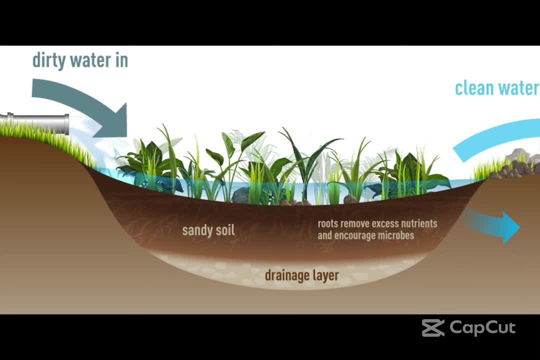 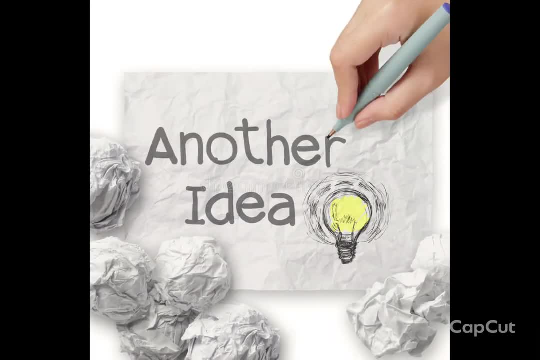 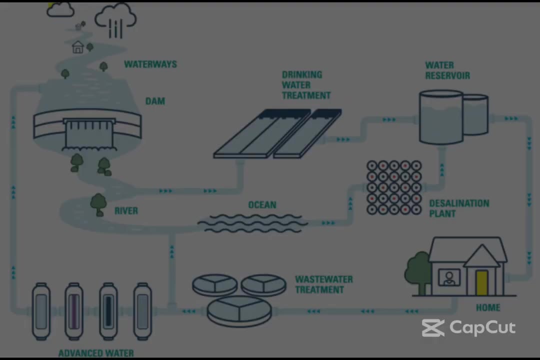 the soil on top acts as a filter. Groundwater is usually free of micro-oil micro-organisms that may cause diseases. Another way to improve Eritrea's lack of fresh water is to save and recycle the water they use. Eritrea can recycle the water they use for showering, cleaning and cooking.